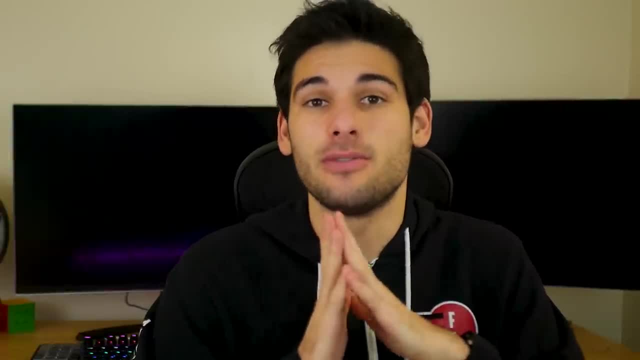 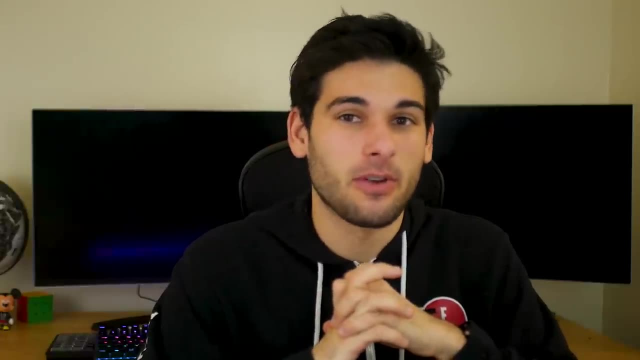 there are actually some things you can buy that are designed to conveniently be good for your privacy and security without much work, which is pretty cool. This video will take you through some of our favorite products you can buy designed to benefit your privacy and security. 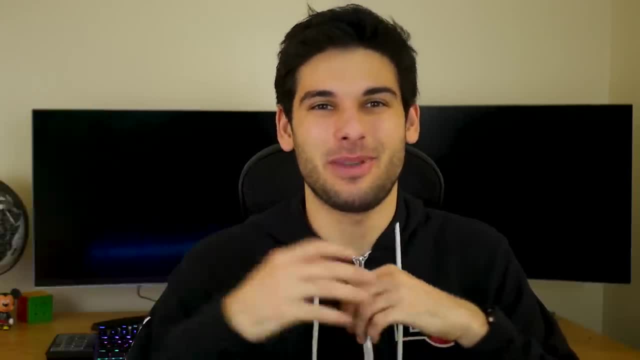 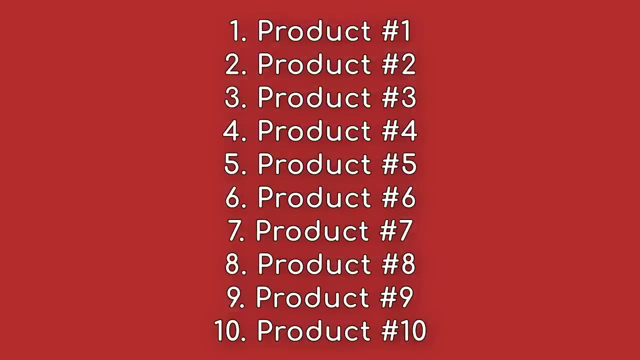 some of which are advertised to do so And well, others may have some inspiration from MacGyver. We have 10 products for you, in no particular order. We'll leave links in the description for all products mentioned. These links will benefit us at no cost to you, but feel free to. 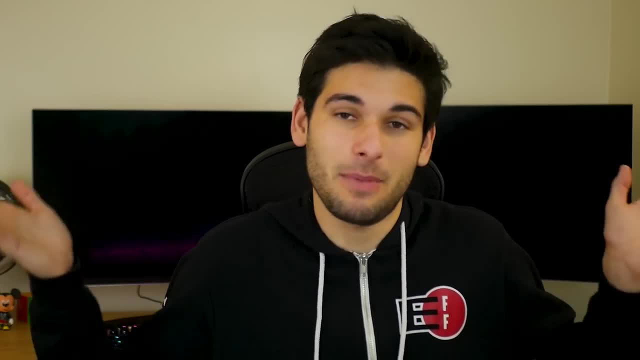 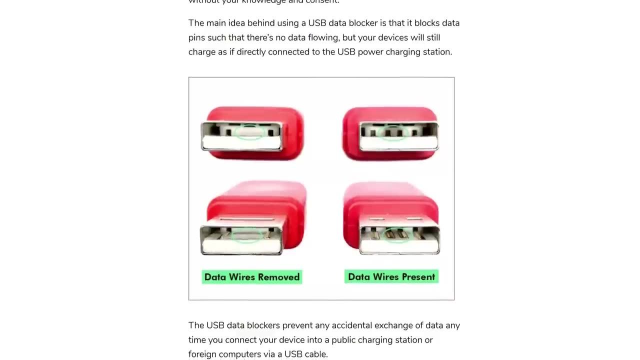 get these products through other means. If you don't want to support us, we'll just be happy to know you got them. Product number one is a USB data blocker. These work by removing the data prongs from the USB interface, which allows you to charge your device but removes the possibility of data flow When 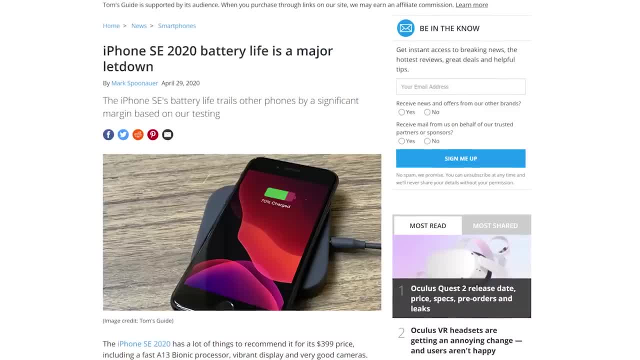 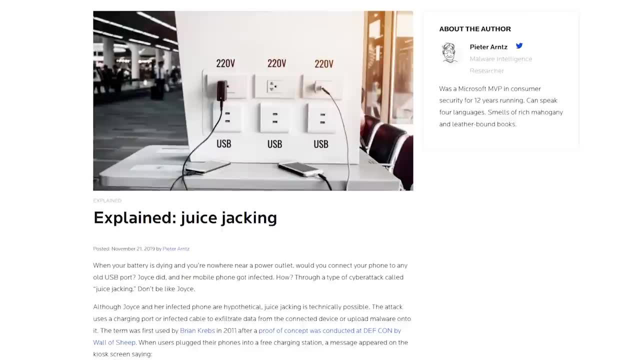 you're traveling through airports and hotels, especially with your crappy battery, there is a small possibility. you could be victim to something called juice jacking, a method of either stealing data or loading malware onto your device from an infected charging port At the Wall of Sheep. 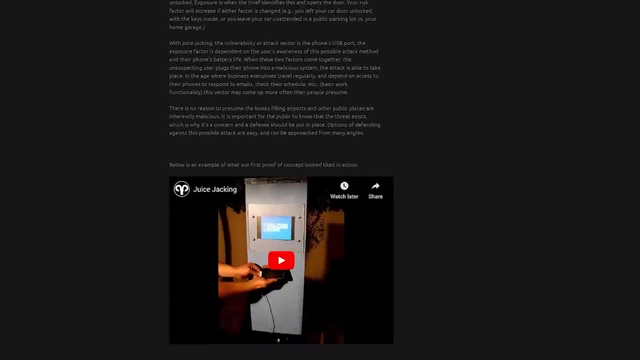 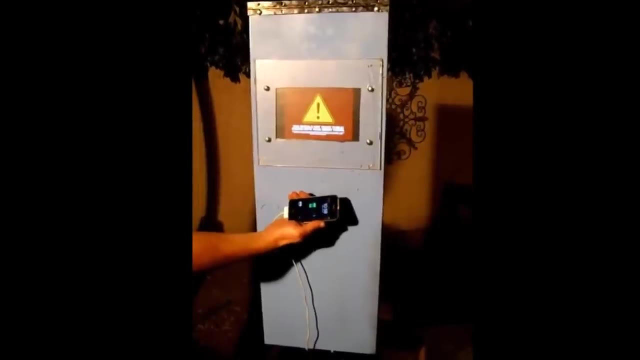 an event at DEF CON, they gave public access to an informational juice-jacking kiosk. These included a hidden CPU which was used to notify the user that they should not plug their devices into public charging kiosks. iOS and Android have taken some mitigations. 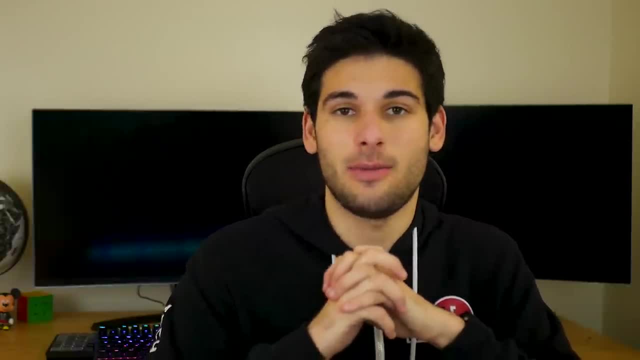 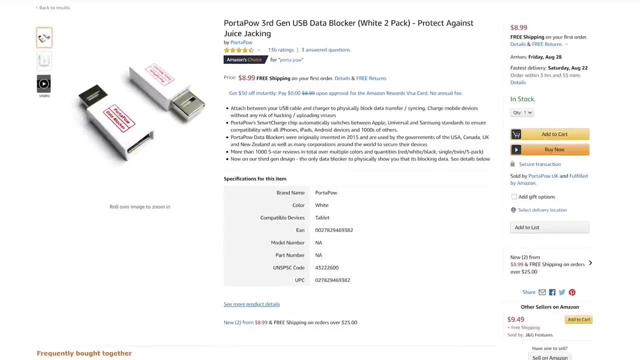 against this, but they are software workarounds. If you want peace of mind, USB data blockers are a guaranteed way to stop all data flow through USB. It's cheap, fits in your pocket and will offer great peace of mind in public charging spots. 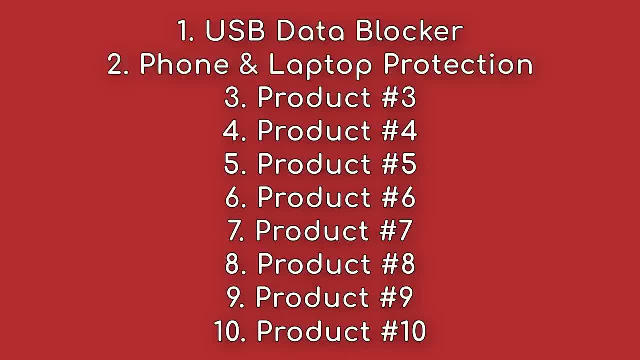 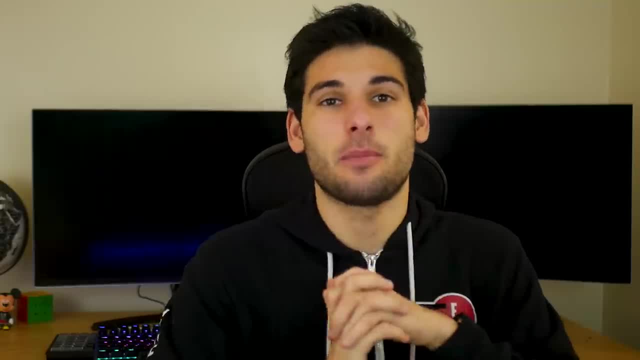 To continue in the mobile space. product number two is a collection of products we recommend for your phones and laptops, The first of which is a privacy screen protector. These make it hard for people around you in public, or even your nosy friends, from peeking at what you're doing from. 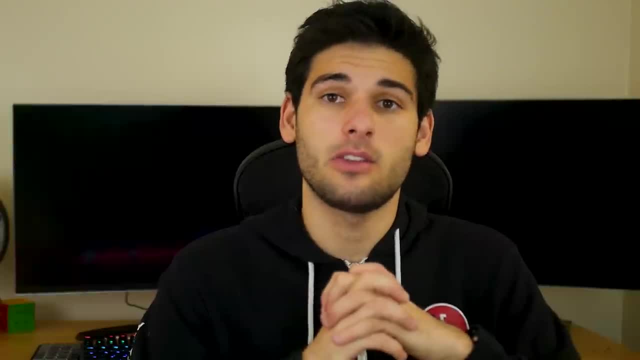 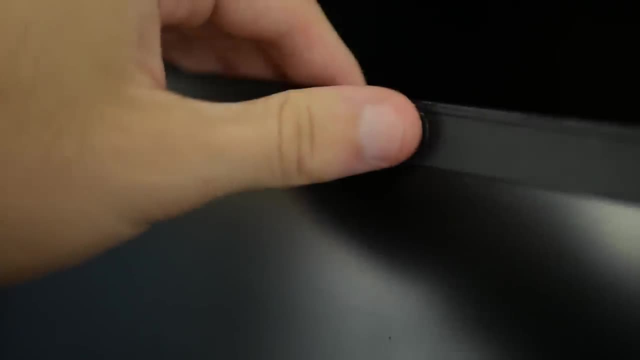 sight angles. Once you have one, you'll never go back. The second is a webcam cover to prevent unauthorized access to your camera. You can get sliding covers for your front camera or just put tape if you never use it. There are also some sliding case covers for rear cameras, depending. 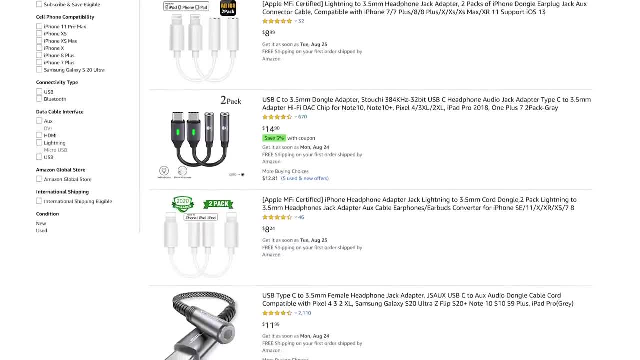 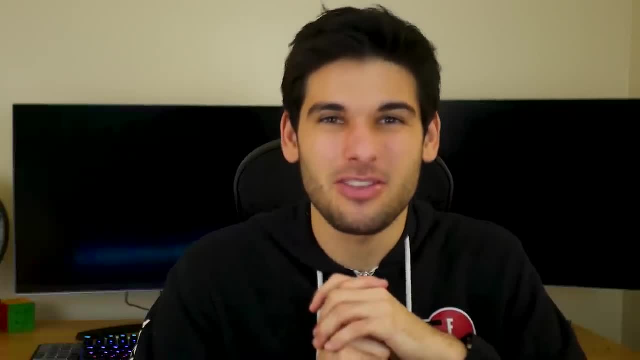 on your phone model. Lastly, we recommend a 3.5mm audio jack for those of you without a 3.5mm audio jack to avoid using Bluetooth, which is an inherent security risk. It's important to use protection, especially with strangers. 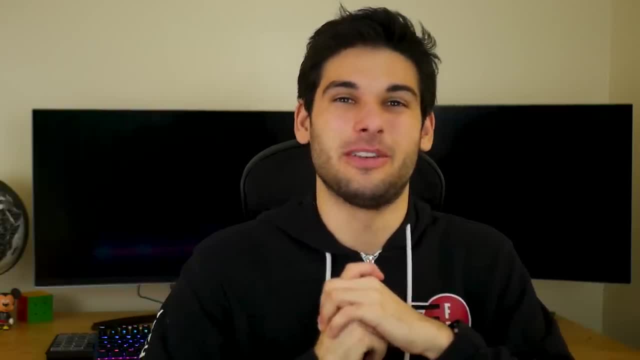 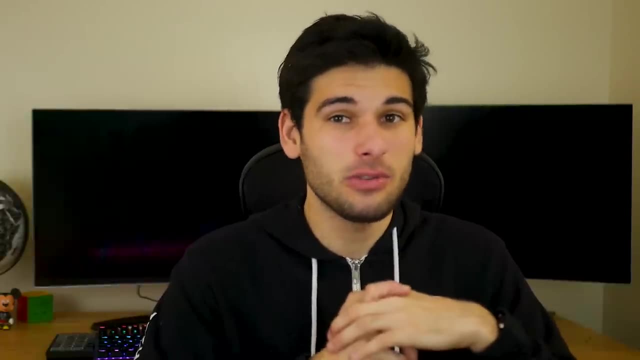 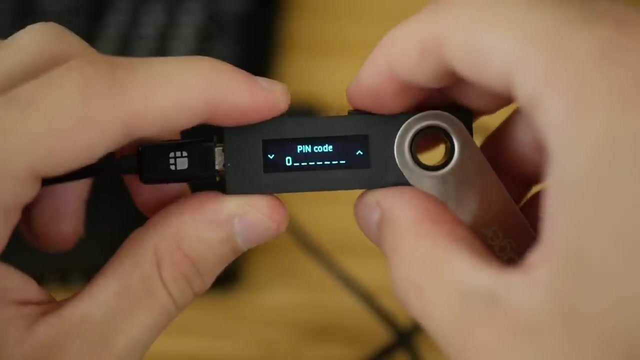 Carlos Matos may be what you think of when you hear the term cryptocurrency. I'm here to tell you cryptocurrencies have valid use cases and hardware wallets are a fantastic and secure method of storing them. We highly recommend the Ledger Nanos. They are simple. 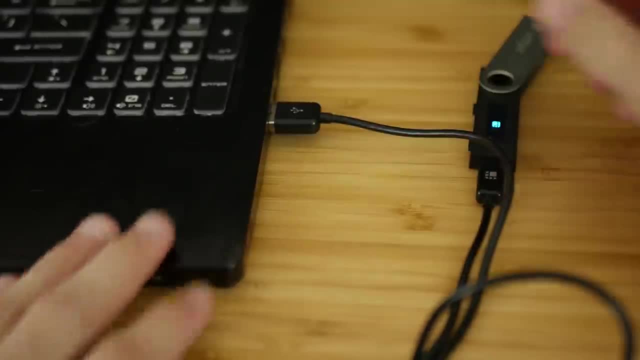 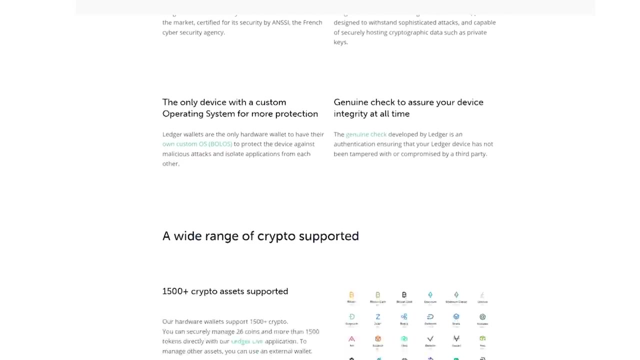 convenient and secure, which is a pretty rare combination. There are some alternatives to the Ledger, but we recommend the Ledger because it's the most tested, an excellent go-to option and a staple in the industry, all for a relatively affordable price. 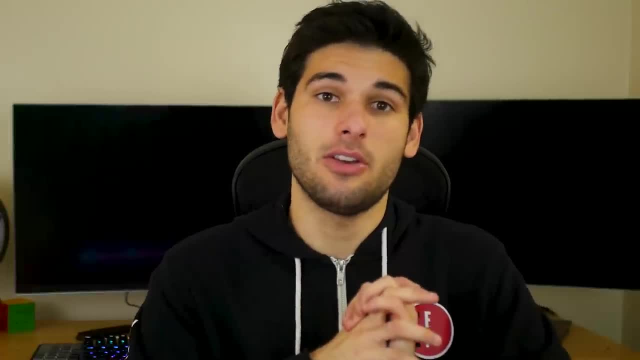 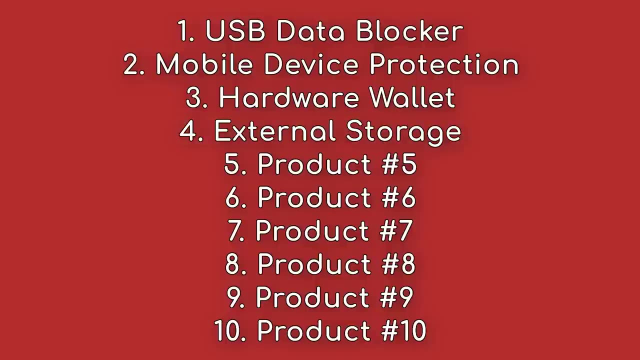 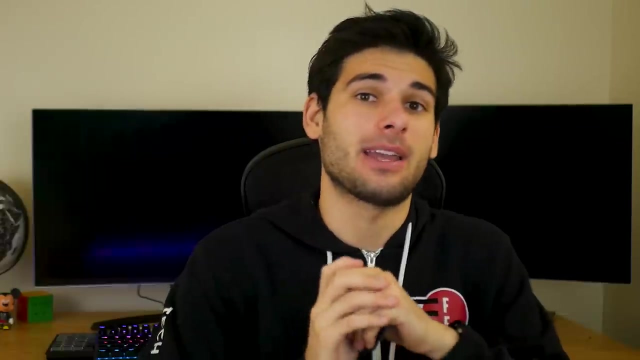 Now, not everything needs to be built for strictly privacy and security. for us to repurpose things a little bit, Product number four is external storage, and we have two recommendations for you. The first is an external hard drive, or SSD. We recommend these for backing up your data and transferring data on the go. 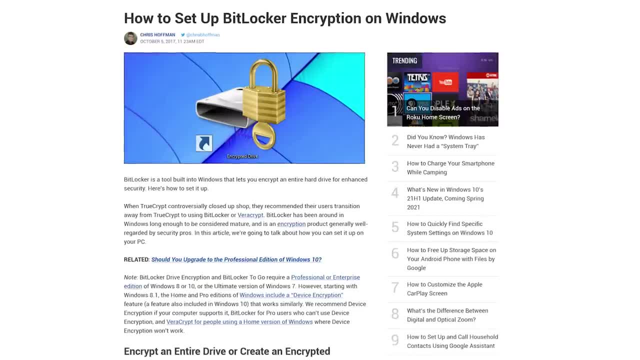 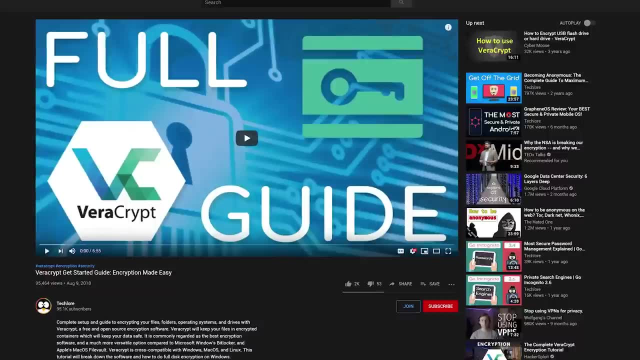 Where this becomes a security tool is when you use VeriCrypt or another encryption software to encrypt the drive, removing the need for you to store your data on the cloud or other insecure methods. We have a guide showing how to use VeriCrypt and if you have an external drive. 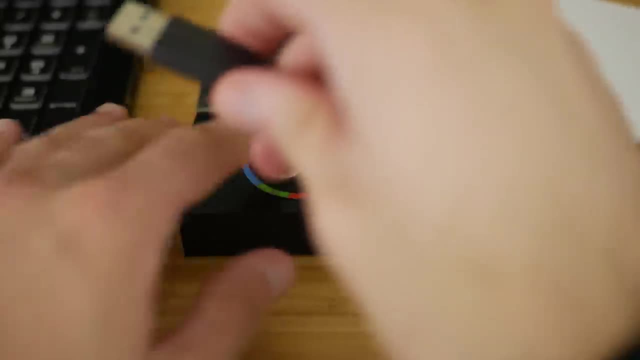 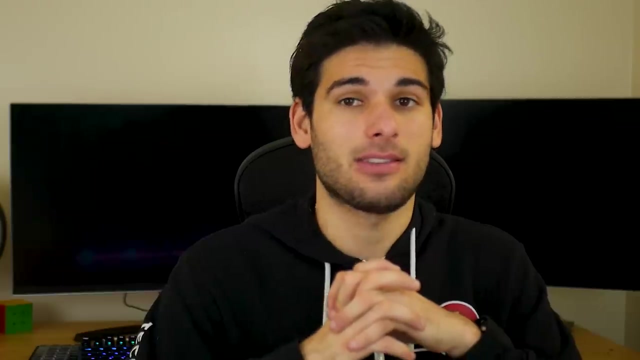 those instructions will enable you to carry your data anywhere with the peace of mind that if you lose the drive, no one will likely be able to break into it. Similarly, flash drives are a great tool for the same exact scenario. but another cool perk to flash drives is they are great for: 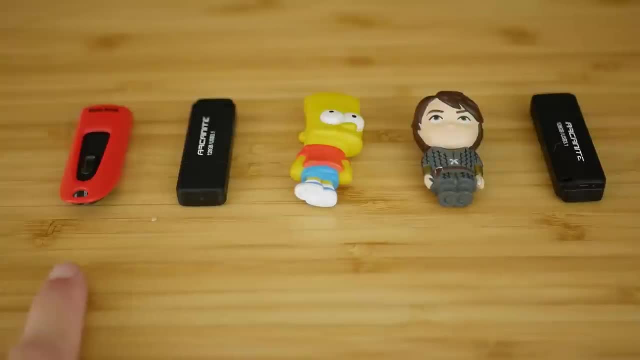 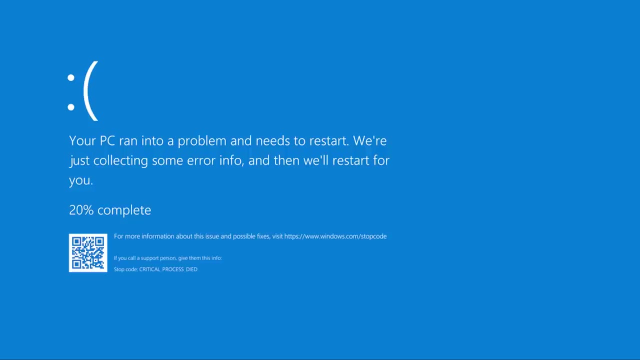 manufacturing systems. Both myself and my editor carry around several flash drives in our backpacks, each loaded with different operating systems like Tails OS, a recovery Windows ISO, because you never know when you're gonna need that one… and more, You can have an OS Arsenal. 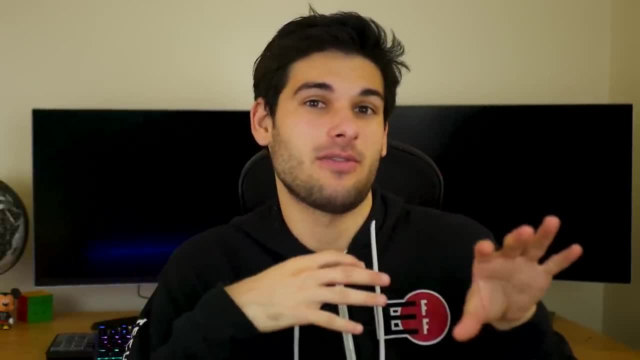 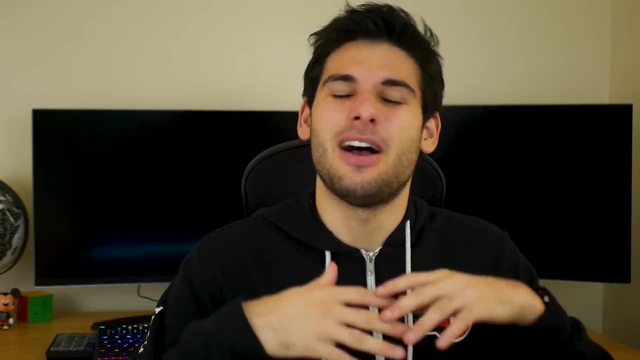 it's pretty freaking dope. Another layer to this is you can have a flash drive with your keypass database. watch our video on Keypass inside a VeriCrypt container if you wanna go that far. That means you can boot into any OS on any computer and just plug another flash drive in. 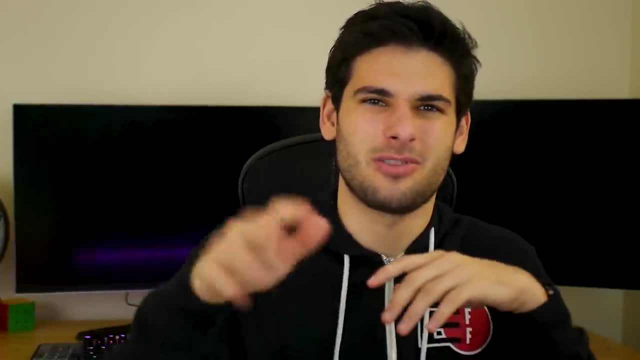 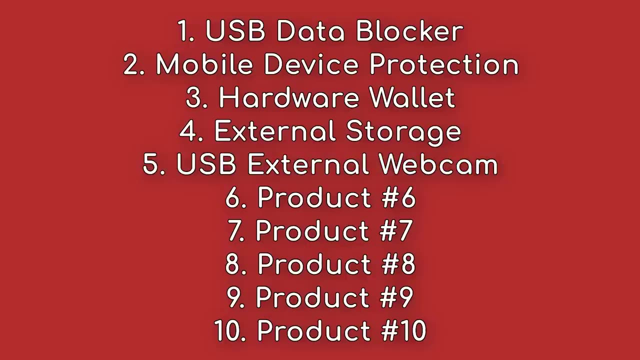 to all of your accounts. The possibilities are endless, so let your imagination run wild. Product number five is another repurposed device. so imagination time. A USB external webcam is a guaranteed way to physically unplug the camera when you're done using it. 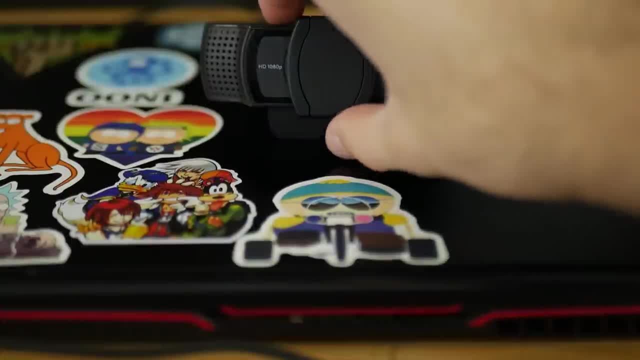 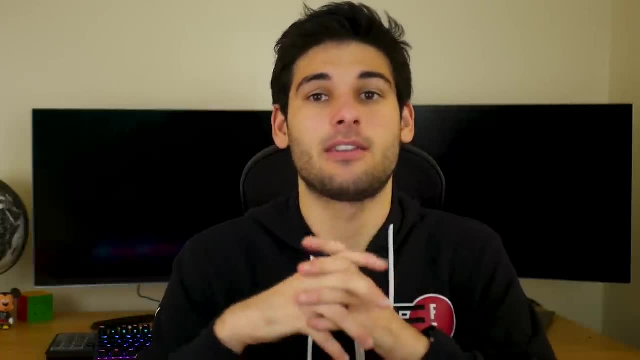 to prevent unauthorized access. Using an external webcam will also allow you to permanently remove or tape up your normal cameras without FOMO. Similarly, we recommend using external mics found on things like earbuds, which would enable you to remove all the mics. 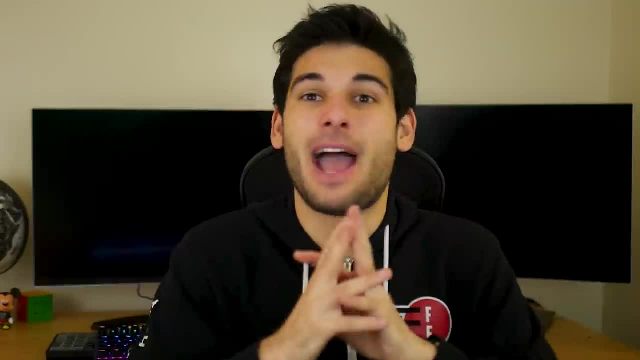 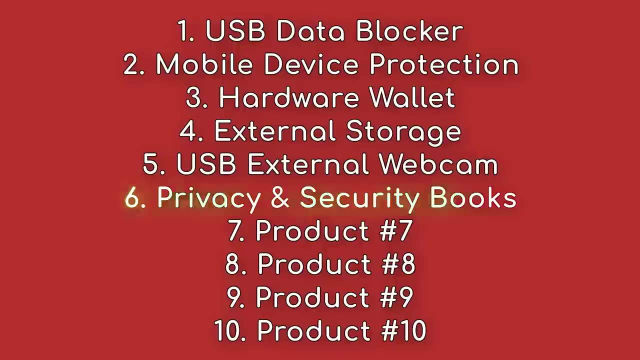 on your devices as well. Knowledge is power, and we believe that constantly learning about privacy and security is just as important as some other things on this list. We have a catalog of our favorite privacy and security books on our storefront. The two biggest recommendations I can make. 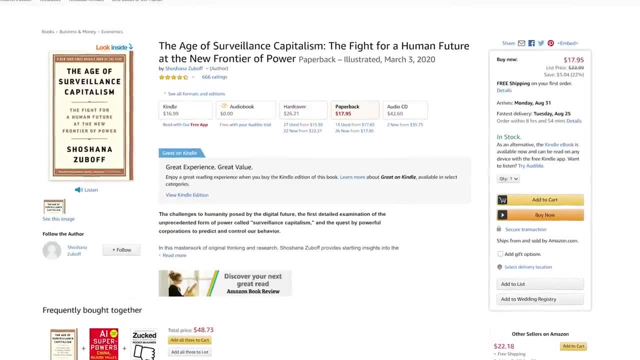 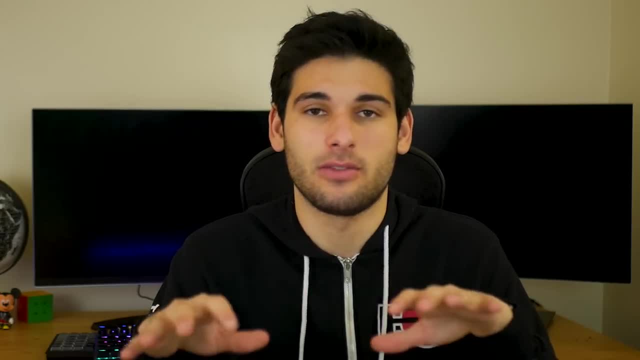 are The Art of Invisibility as well as The Age of Surveillance Capitalism. Seriously, we cannot recommend some of these books enough. They will change your entire perception of how you view the world and what it means for privacy and surveillance. Plus, you'll have bookshelves, just like Tai Lopez. 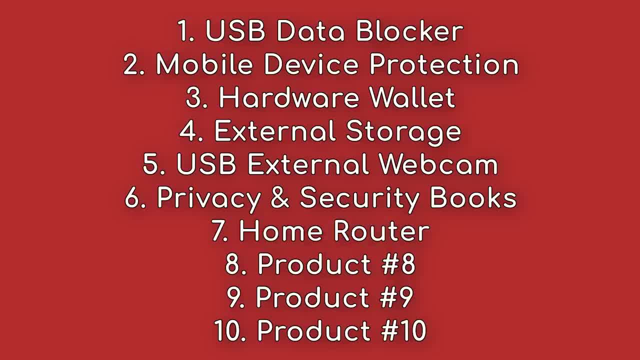 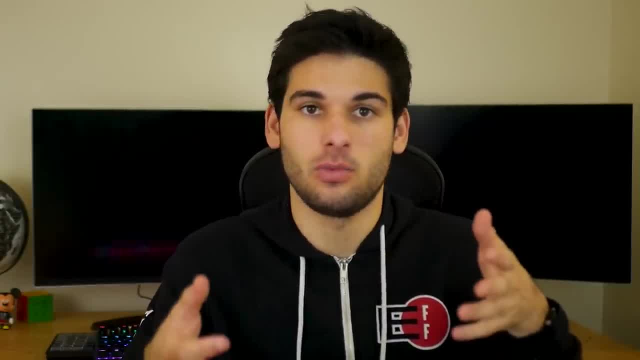 Seven New bookshelves. Your home router may be one of the most overlooked devices you do not think about. The reality is, all devices are connected to this one central device, which has been known to be targets of attacks and are prone to vulnerabilities. Because of this, we recommend picking up a router that supports custom firmware, built for your privacy and security in mind, something like OpenWRT. A very commonly recommended router compatible with OpenWRT is the Netgear Nighthawk R7800,, which people just seem to absolutely love. 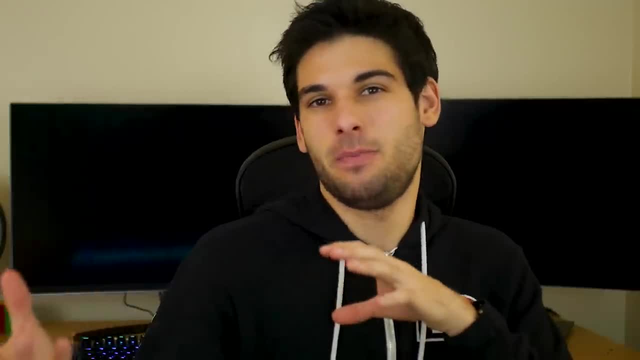 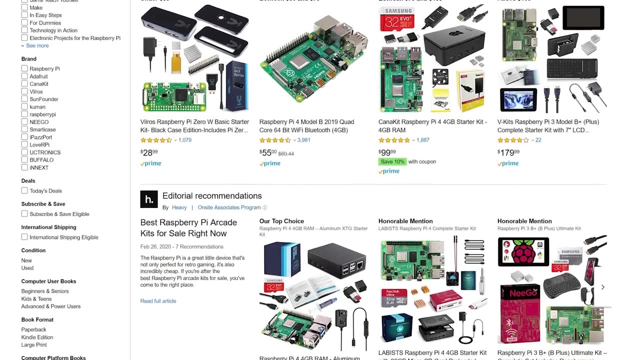 So that's our main recommendation. Product eight is a bit open-ended and it's kind of the DIY zone. We recommend picking up things like Raspberry Pis, looking through DIY projects and seeing if anything speaks to you. Maybe you use a Raspberry Pi as a home storage solution. 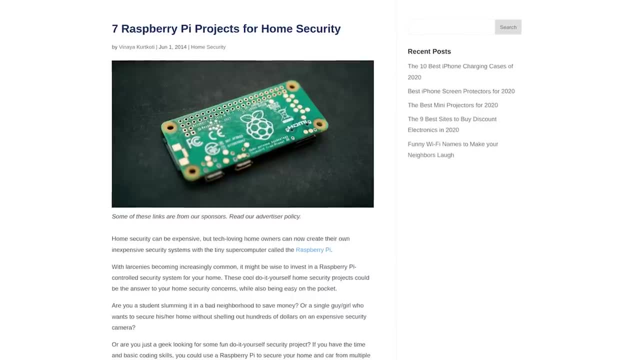 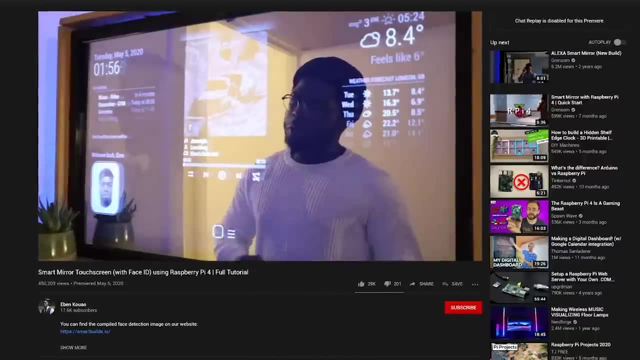 to avoid cloud storage. Maybe it functions as a home security camera hub so you can get away from the stupid Amazon nests. And there are even things like firewalls and intrusion detection systems and I'm sure you can set up some fancy Tony Stark thing. 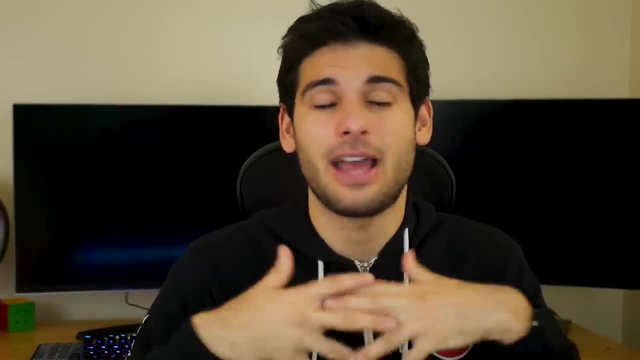 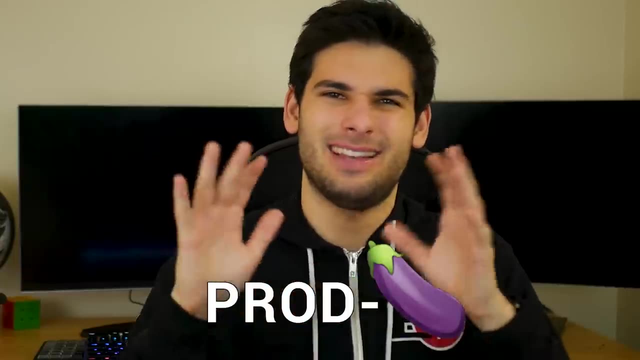 You can do whatever you want. The possibilities are endless and if you're creative, just have some fun with it. Products number nine have prod Products. What is that? Prod-dics? Prod-dics number nine. First, that was awkward. 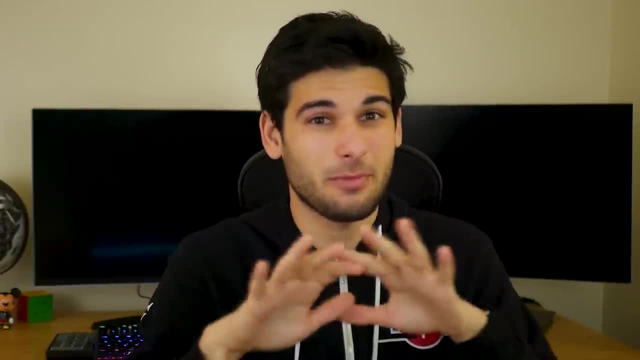 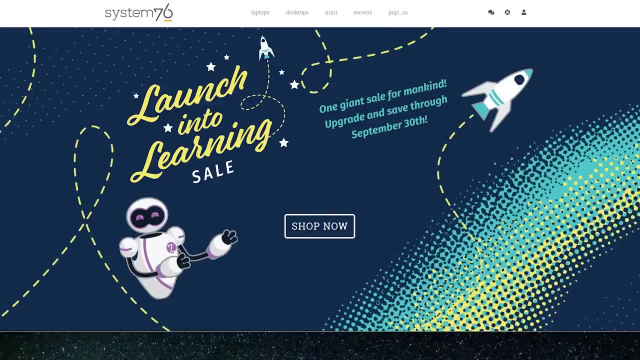 Products number nine have some things that are a bit unpopular in the privacy community. but seriously, please hear us out. First. you can always pick up some of the products from people like Purism, System76,, Star Labs, Pine and other Linux-based manufacturers. 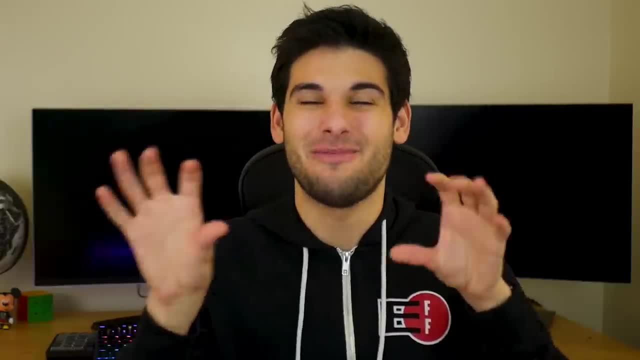 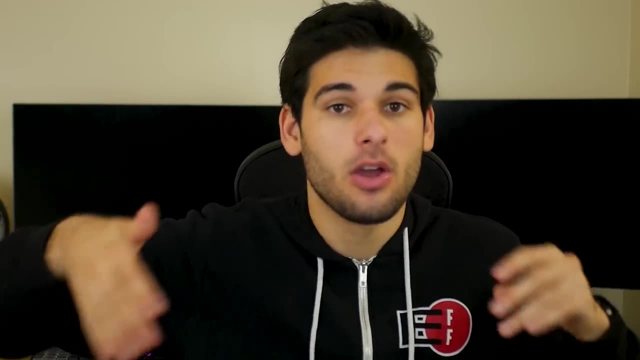 These are all cool projects that have a place. However, it's a better option if you want something with the utmost security in mind out of the box, not necessarily privacy. again, security with fantastic software support, a decent price point and incredible convenience. 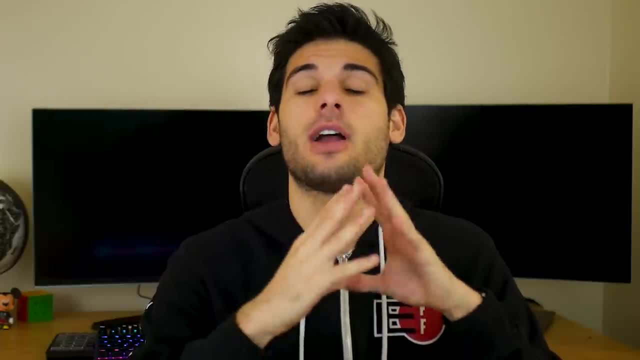 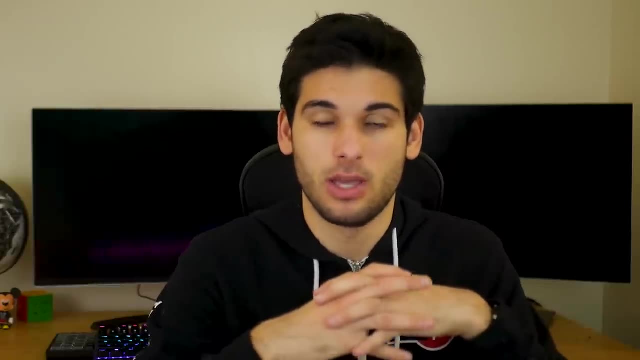 It sounds too good to be true. Again, this is for something that's only for high-security personal tasks, and it's even recommended by Kevin Mitnick in The Art of Invisibility, as well as many modern-day security researchers. The iPad and the Chromebook are both arguably 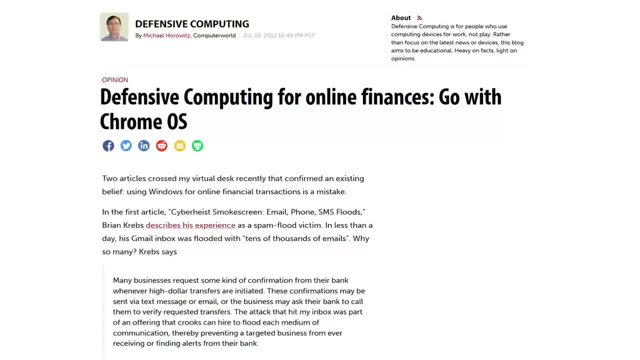 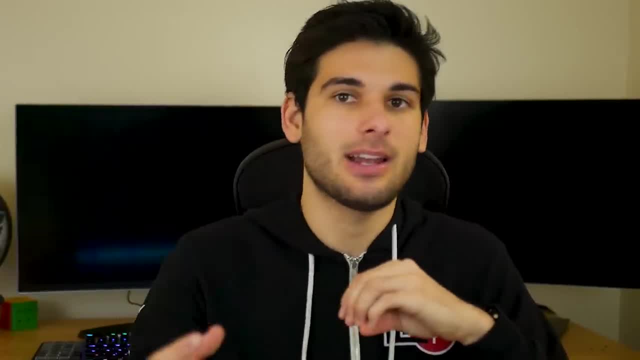 some of the most secure devices money can buy, with some of the tightest sandboxes and security models that protect you from traditional attacks. Yes, they're not open source. Yes, there will likely be data collection from Apple or Google, but again, this is simply for high-security personal usage. 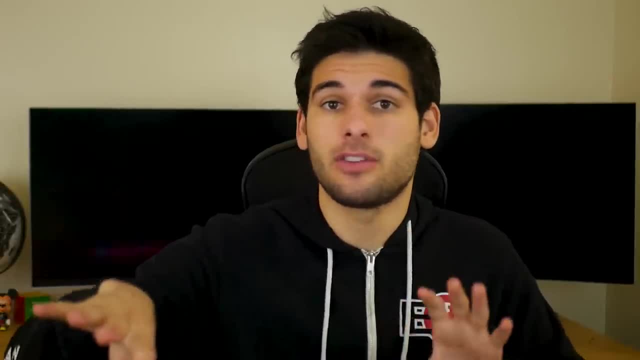 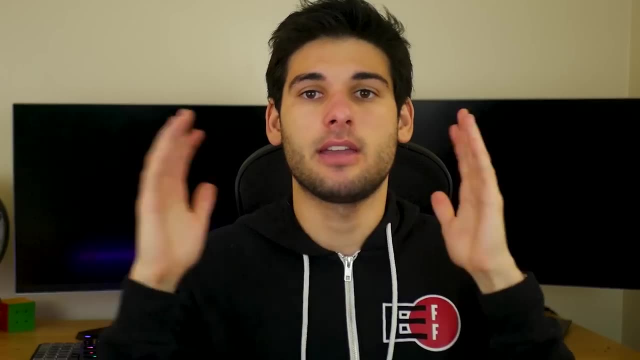 which can be compartmentalized from other activities. These really are some of the most secure devices you can buy and, if you're able to work with that threat model and that's something that you can benefit from, it actually is a pretty sweet setup. 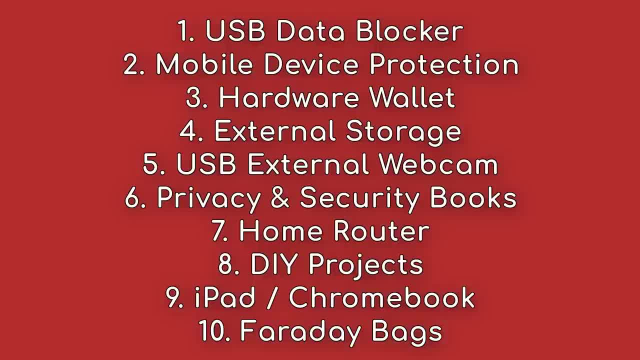 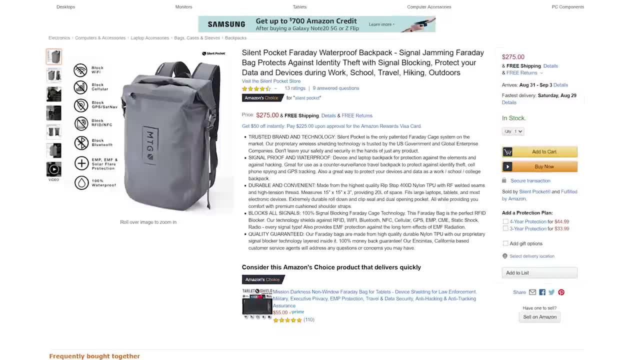 And finally, product number 10 is Faraday Backpacks and Pouches. These are designed to fully eliminate all radios transmitted by your device to guarantee no signal leaves them. The backpack will protect everything inside of its pouch and there are smaller pouches. 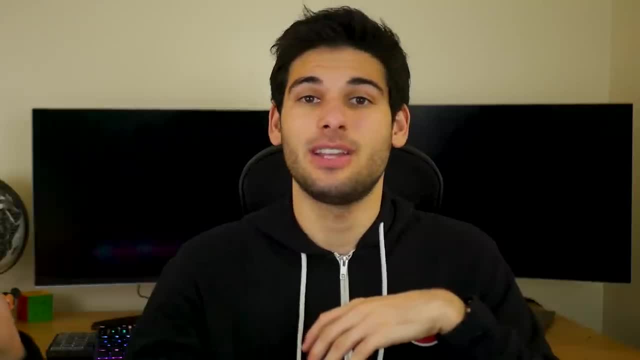 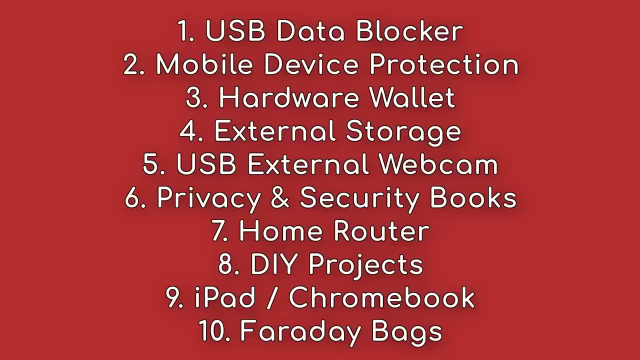 for just your phone or car keys. You can use these when traveling to add hardware-level restrictions if your threat model calls for something this advanced. And that is our top 10 list of products you can buy today, designed or easily modified to improve your security and privacy. 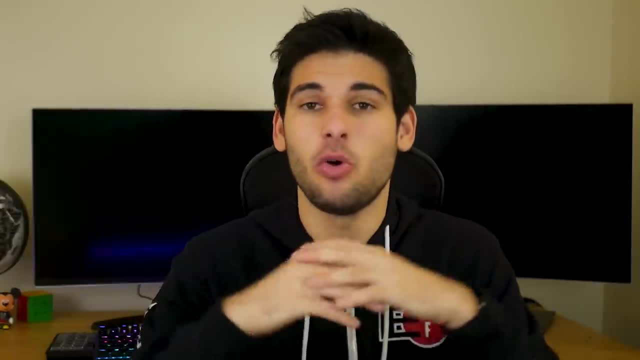 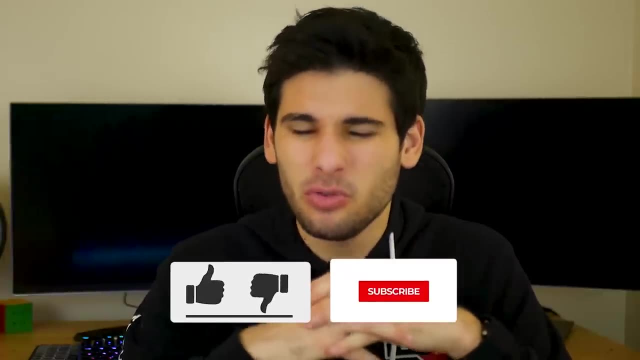 Again, don't forget to check them out in the description. Those links will help support our work, so thank you in advance. if you go through those links, Make sure to leave a comment below with your favorite products that you love and especially, remember to like and share this video. 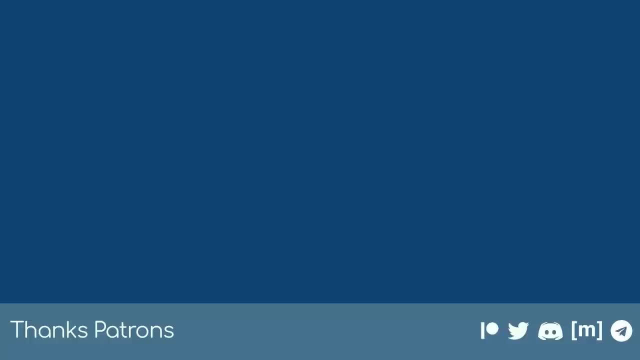 with your friends and family. Thank you for watching and we'll see you next time.